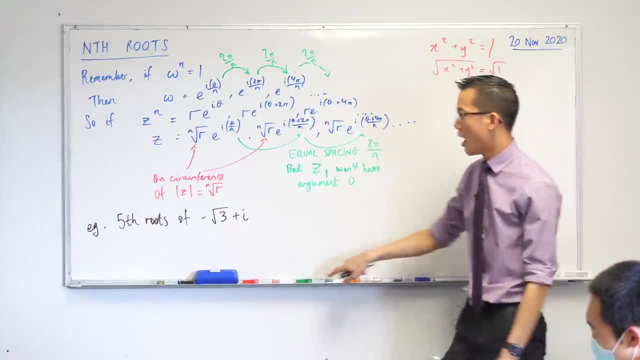 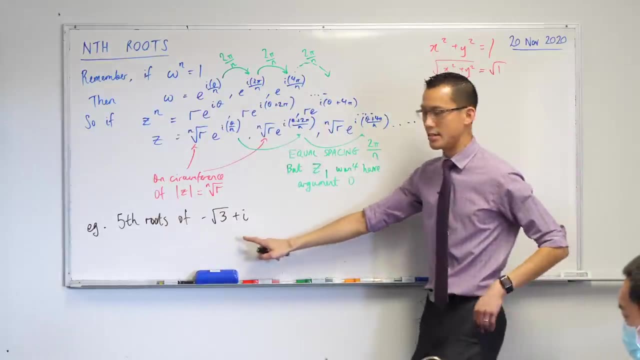 to need to make some space, but I'll give you a minute to write this down, if you're still catching up. I want you to jot this down and think about how we're going to form an equation with our fifth roots in it, if this is our particular complex number. I'll give you a clue. All of 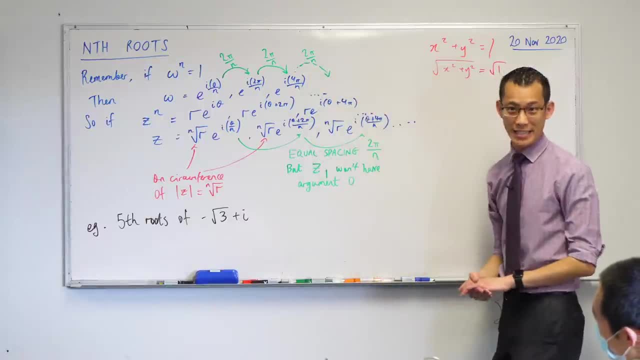 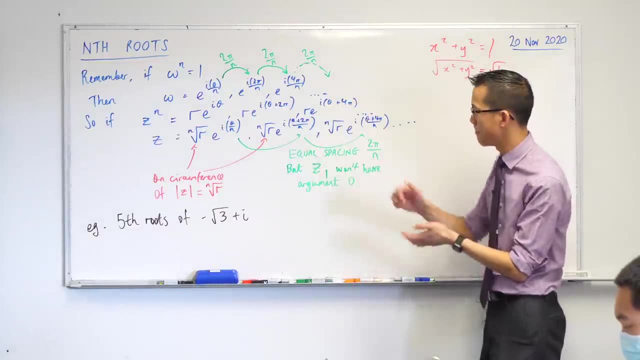 this working, except for the first line, is not in rectangular form, So the first thing you're going to have to do is get things in an appropriate shape to start doing this working. I'll give you a minute or two head start, and then I'm going to clear this off, and then we will. 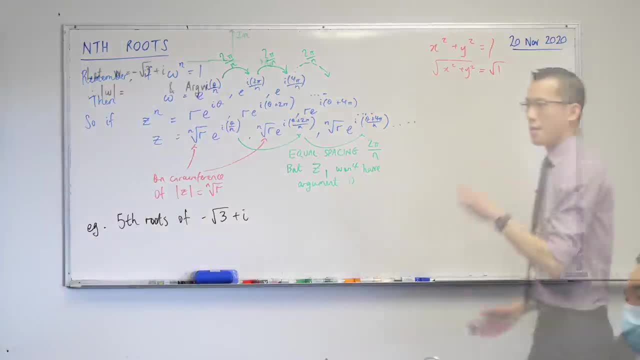 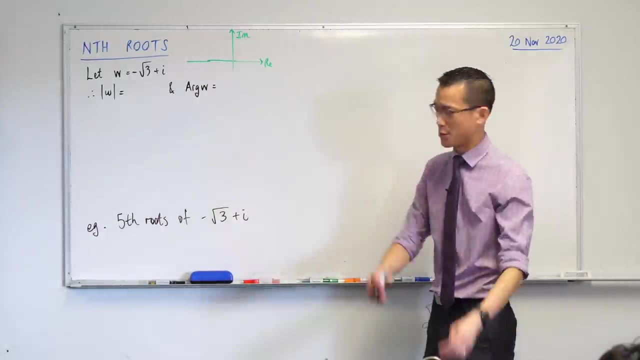 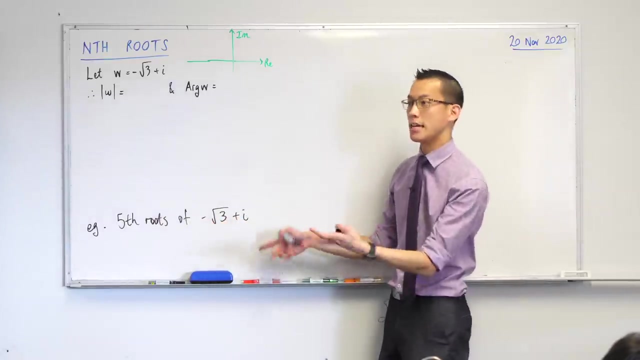 have a go together. Off you go. I can see some people have made a good start. For those of you who are still not 100% confident, let me give you a bit of a nudge. So we're looking at the fifth roots of negative root, three plus i, which is given to you as it often will be in rectangular. 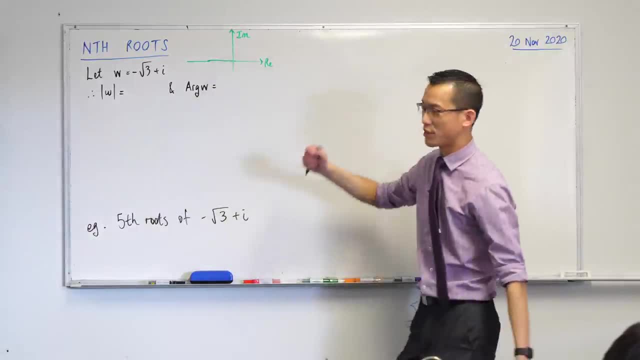 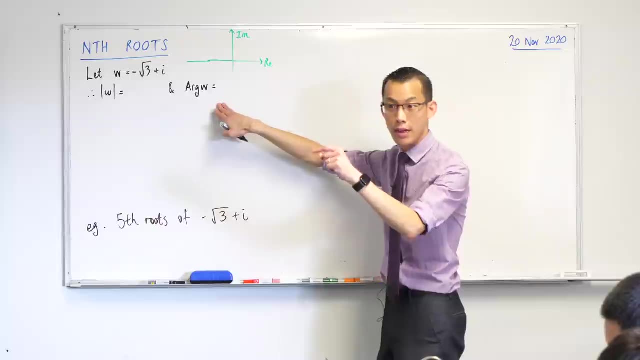 form, But rectangular form kind of sucks for finding nth roots. So the first thing I'm going to do is work out what the modulus is, what the argument is, and then I can go into exponential form. So real quick you'll get to the point. you actually saw me doing this live when I was trying. 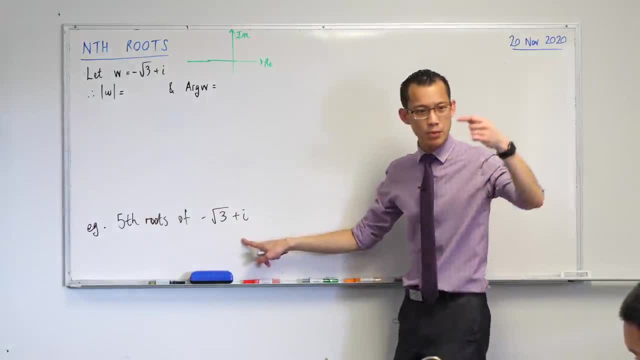 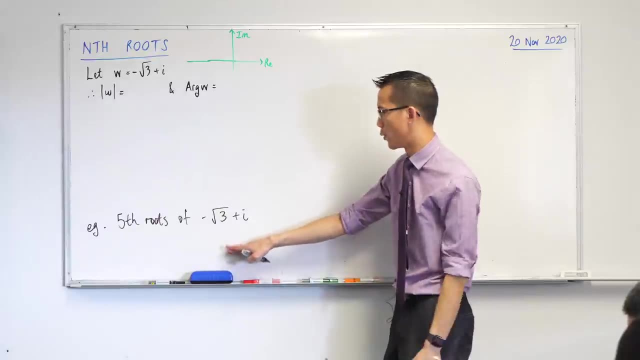 to remember. if I got this question, this particular number, right, You'll get to the point where you're like, oh, I can visualize, especially because these same numbers to give you exact values- will come up over and over again because we don't want to make it a pain for you. You'll start to think. 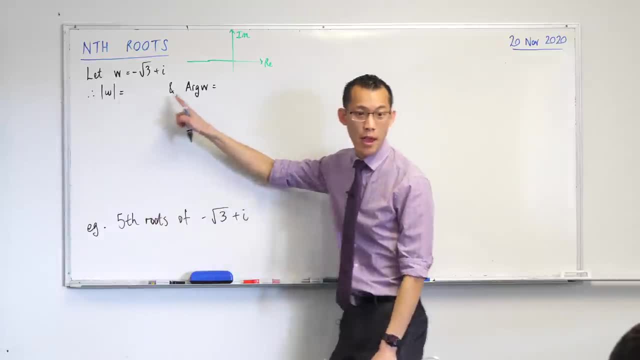 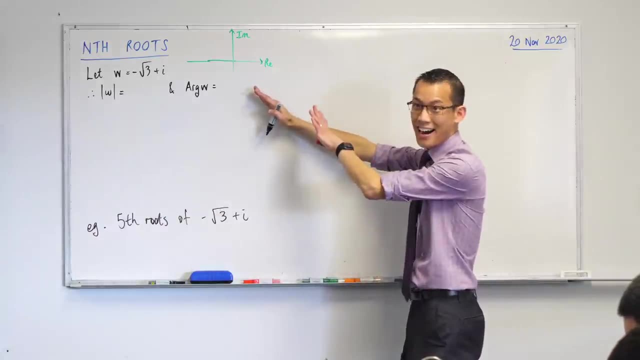 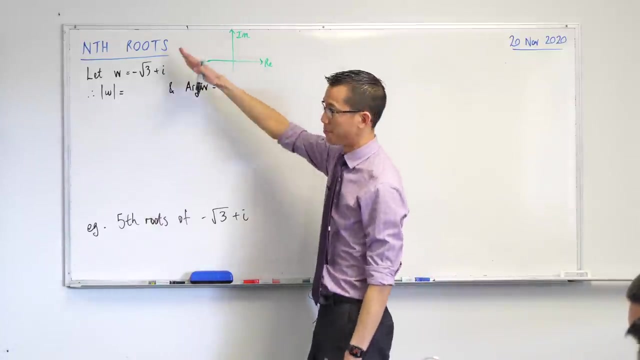 oh, I know where this number is, so I can quickly verify what my modulus or my argument should be. So I'm going to draw myself a favor: Draw yourself a tiny little Argand diagram and think about where this is going to be. Negative root three: that takes you to the left of the complex plane, because 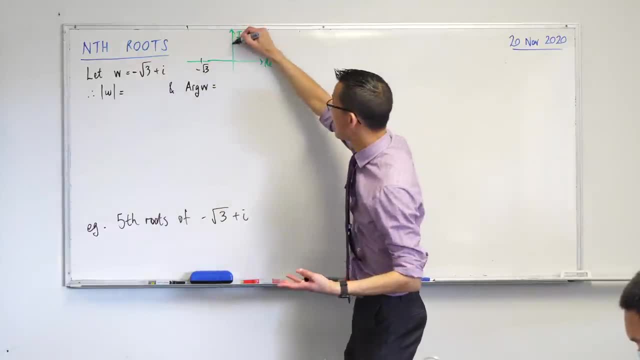 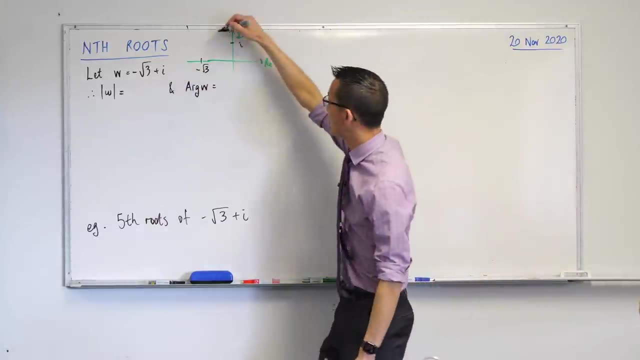 it's negative root three over here, plus i takes you up further into the imaginary axis, but this is one and this is 1.3.. So here is where I would place what did I call it? I'm calling it w okay. 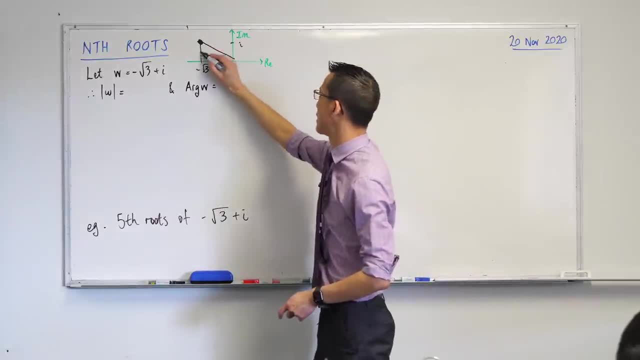 So, if that's where w is, if you have a think about this triangle you create in here, this is our 1, 2, root 3 triangle right: 1, 2,. oops, wrong way around. 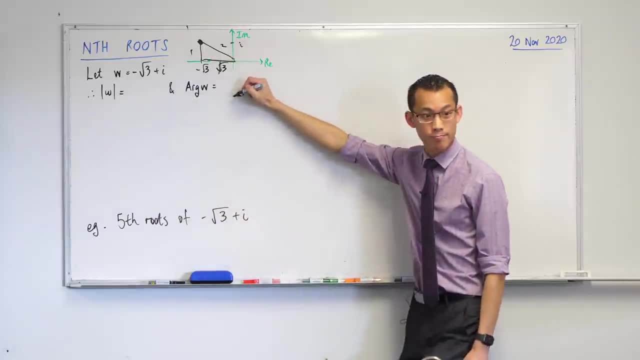 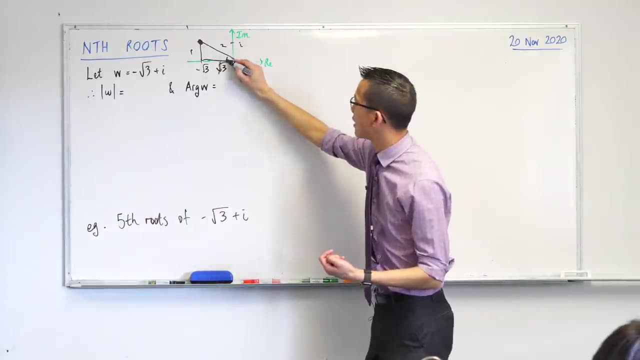 1, 2, and then root 3 on the bottom right. So you're going to get pi on 6,, pi on 3, and pi on 2 in this triangle. You're just going to know which one is which right. This angle here is the one. 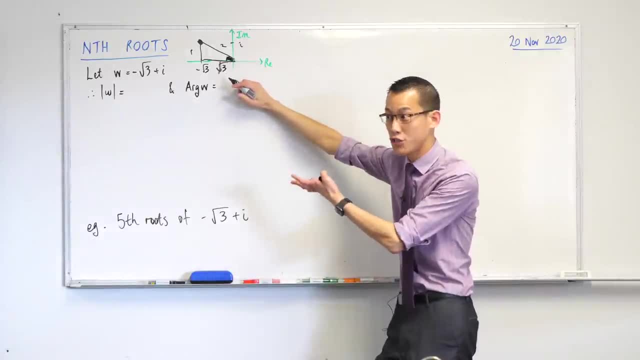 that's most relevant to me. What is the side? You can even see it on my messy diagram. Which angle is that? That's pi on 6. It's the smallest angle, right? You can even see that, just because my scale. 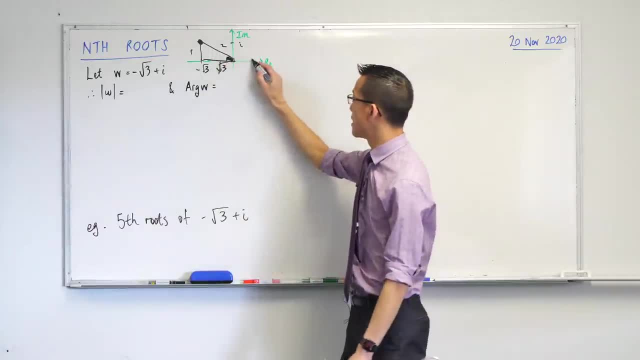 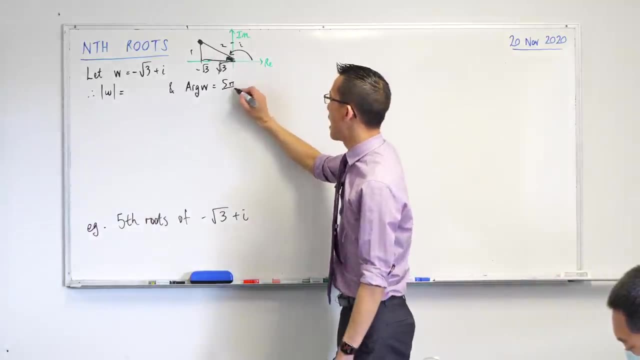 is roughly close enough. If that angle is pi on 6, then the argument that I'm after is the supplement of that. It's 5 pi on 6.. So I'm going to jot that down here, and I kind of sneakily already mentioned this without writing it. 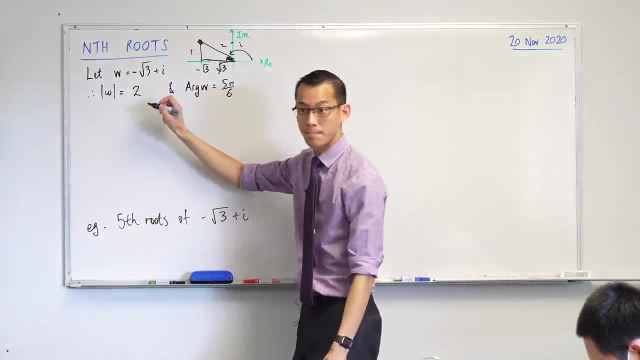 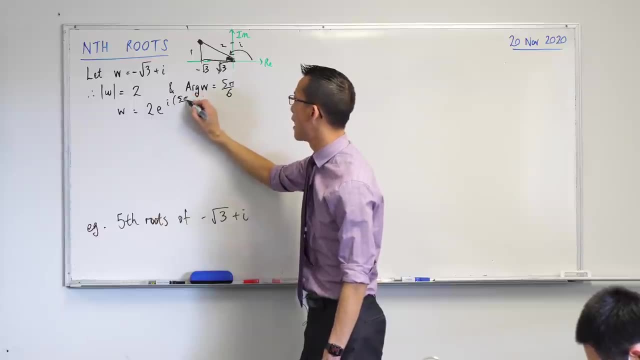 The hypotenuse is the modulus that I'm after, so that's going to be 2,, okay, So therefore I can say w equals 2e to the i, 5 pi on 6,, and so now I'm kind of ready to work out what my nth roots will be. 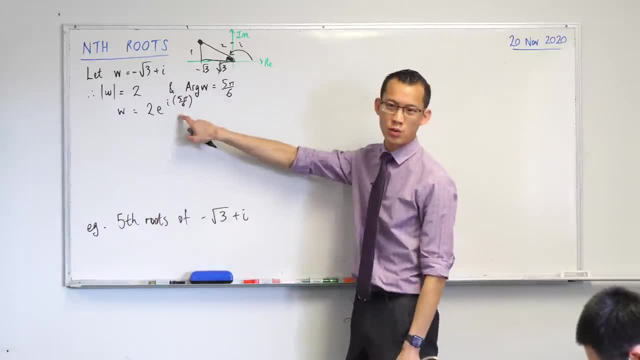 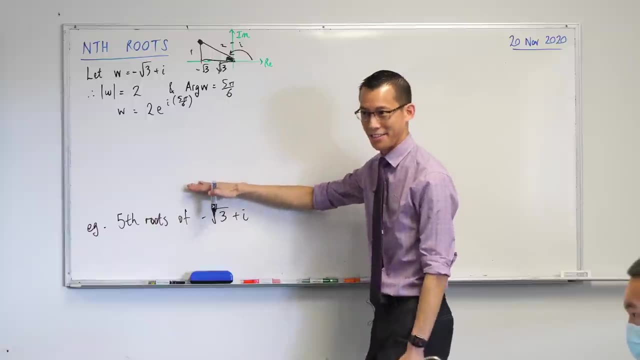 I'm after the fifth roots, right? So I'm going to say I don't just want this, I want, like the 5, sorry, the 4- after this, right? So what I'm going to do to sort of minimize the amount of working that I'm going to put down. 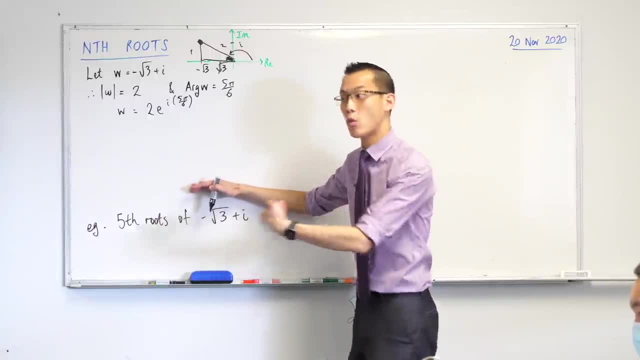 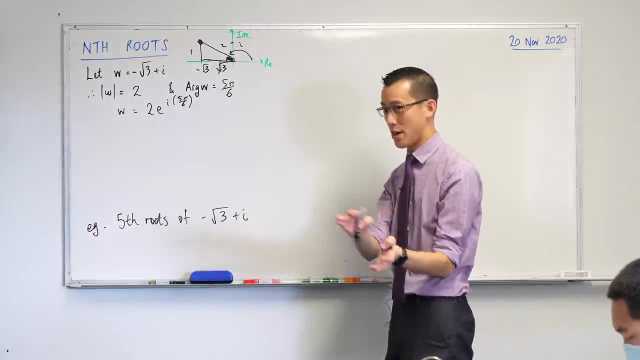 I'm going to find the first solution, what I called before z1, and then I'm going to use my sort of the fact that I know they're going to be spaced around a circle with a particular circumference and just use that to find the rest. 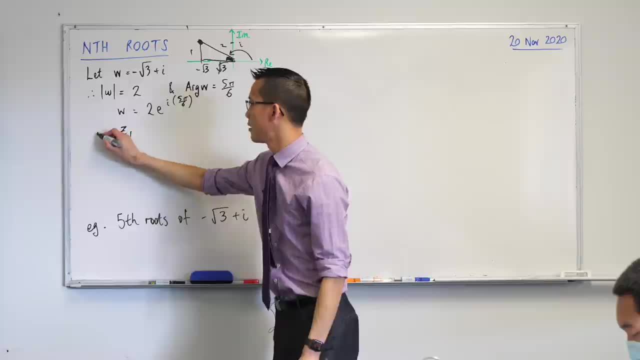 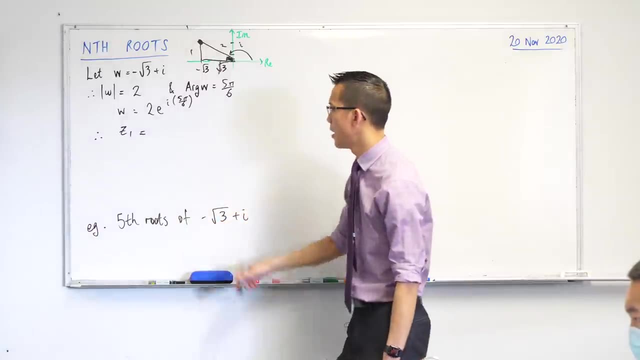 of the solutions. okay, So I'm going to say z1 will be this thing raised to the power of a fifth. Do you agree with that? I'm looking for fifth roots. okay, So when you raise 2 to the power of a fifth, how would you write that? This is just a real number. 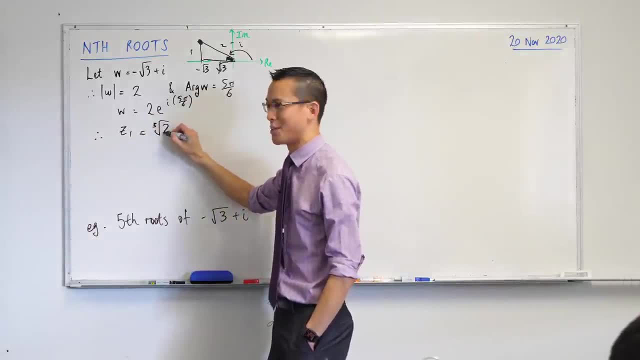 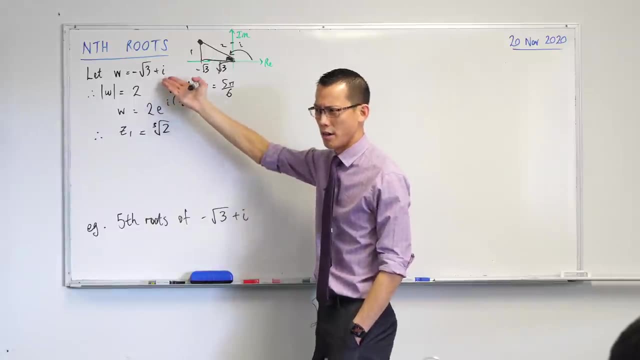 This is the fifth root of 2,, right, Is that? okay, Which is not like. I mean. I've chosen numbers here for you, so the numbers are small. You might have gotten like, say, 32 on a question was trying to make things easy for you because that's the fifth power of 2.. But here, 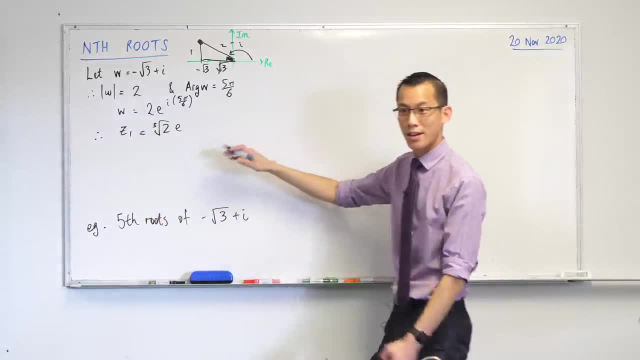 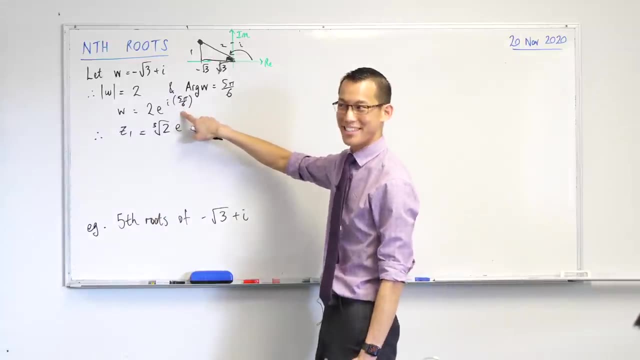 I'm just going to write the fifth root of 2.. Then I come to the the argument part, right? So I'm going to take this and I'm going to divide by 5.. Oh, that's convenient. So I'm going to write i to the pi on 6 up here. 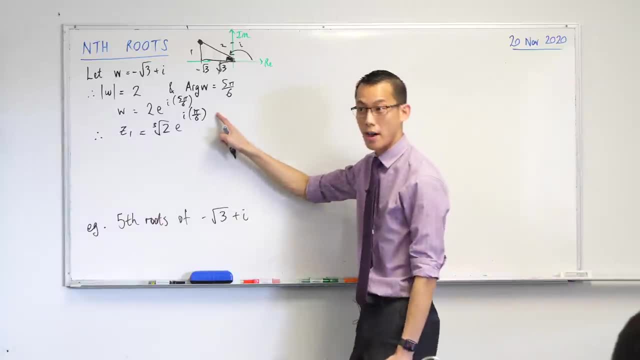 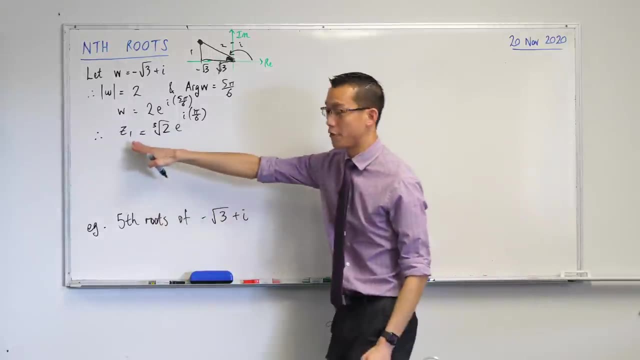 There's my first solution, because I've divided this by 5, okay. So there's my first solution. I need to put some kind of connective tissue here to explain how I'm going to get from z1 to the other roots: z2,, 3,, 4, and 5, okay. 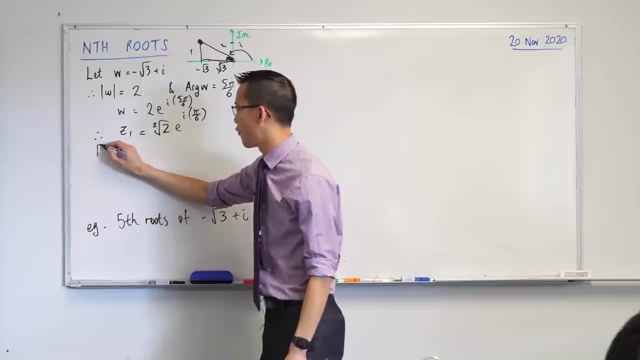 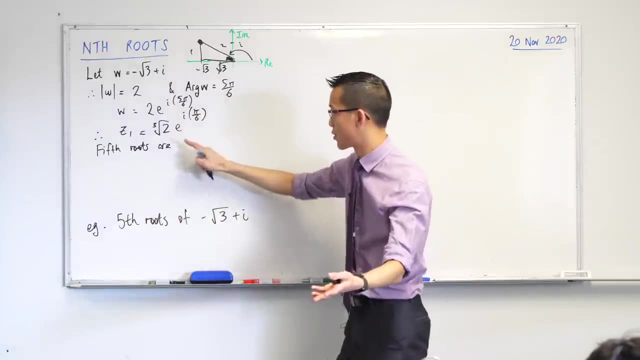 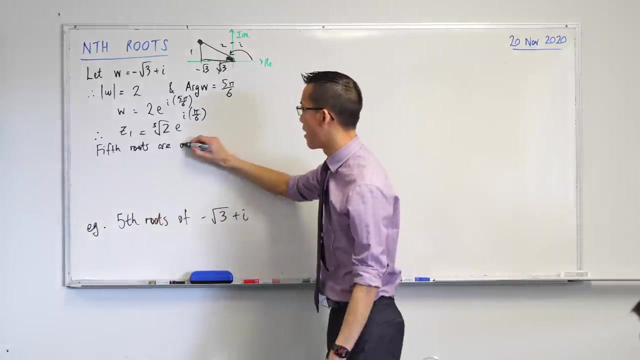 So I'm going to say fifth roots need to include that are on. I'm going to say a circle of circumference, fifth root of 2.. You can say that phrase a circle of circumference, fifth root of 2, or you can say there on the absolute value of z equals the fifth root of 2.. 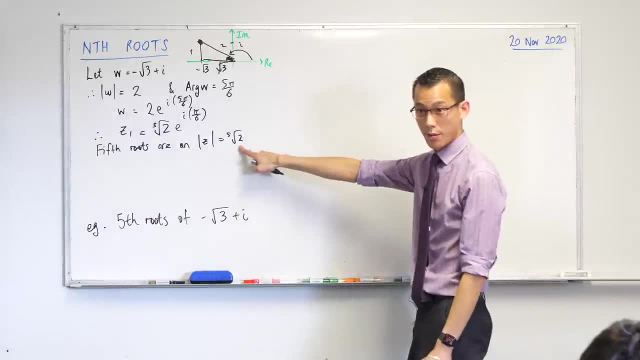 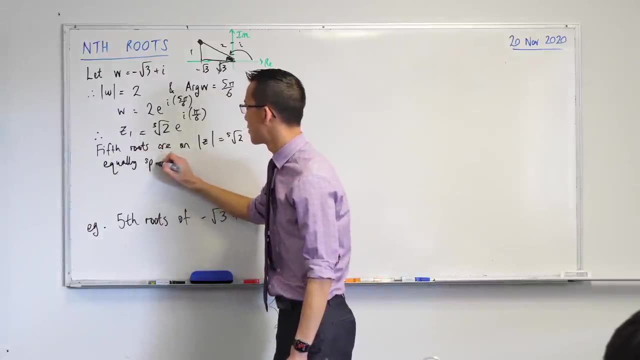 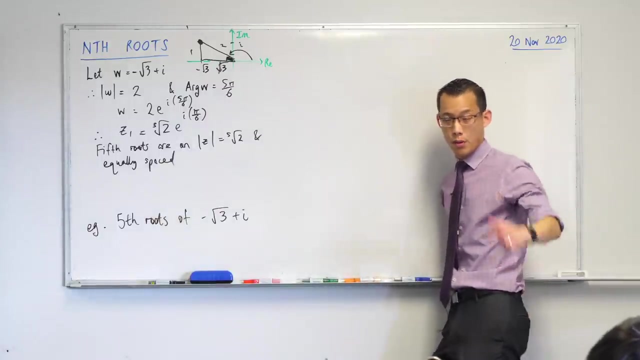 That's another way of saying. this is the circle that has that circumference right And they are equally spaced. What would be the spacing in this case? You can have a look. I've already rubbed it off, but you can have a look at our generalized working before We would say they're. 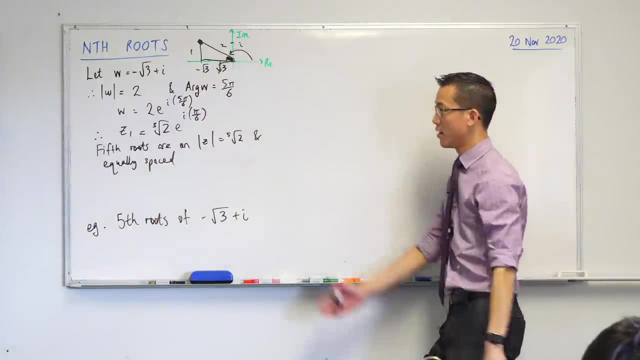 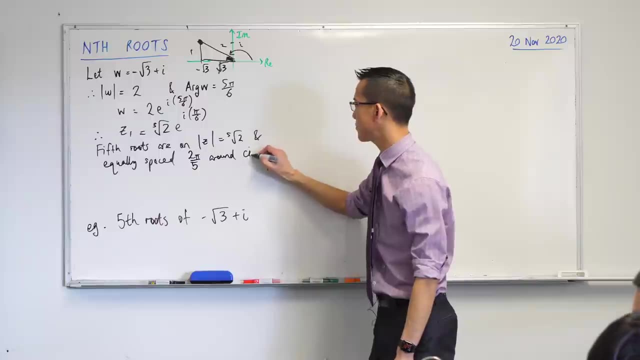 2 pi on 5, in this case 2 pi on n, where n is equal to 5.. So I'm going to write 2 pi on 5 around the circumference. Okay, so this piece of connective tissue, it's really important. 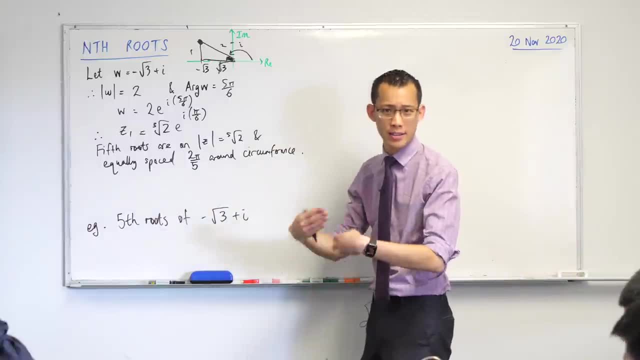 You don't want to just go to like the next working. it's like: where did this come from? okay, As I work out z2,, 3,, 4, and 5,, I'm explaining how I'm going to change this and also I'm going to keep it the same. 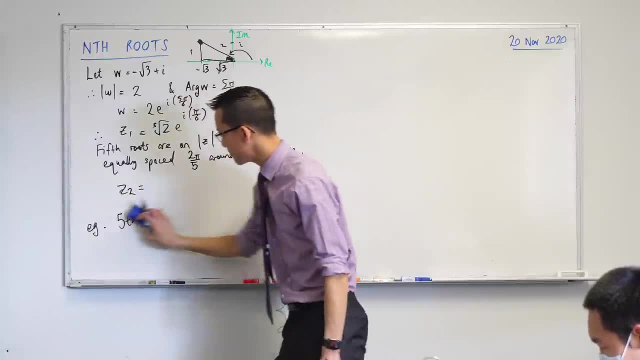 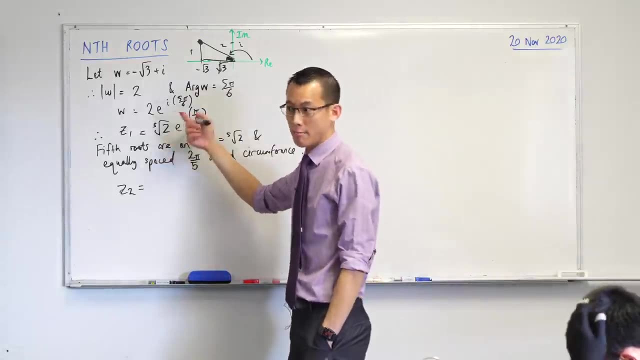 So when I write z2,, for instance, because I know I'm on this same circle- what happens to this modulus for the next solution? Yeah, it's the same modulus. that's nice. Okay, but then you want to have to think about the next solution. 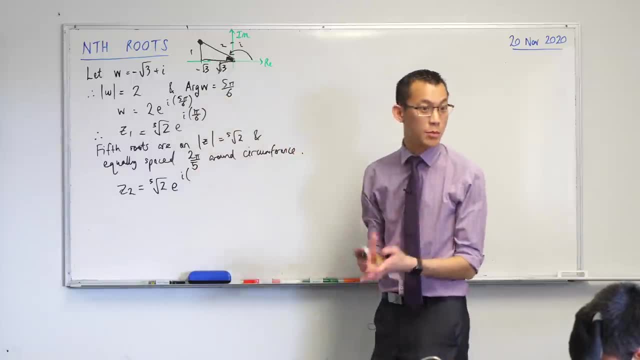 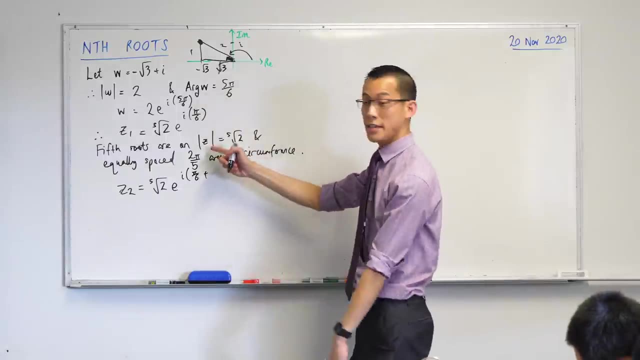 It's going to be e to the i. my angle is going to change. my argument will change. right, You're still going to start here, but pi on 6, you're going to add on what my spacing is, which in this case is 2, pi on 5.. 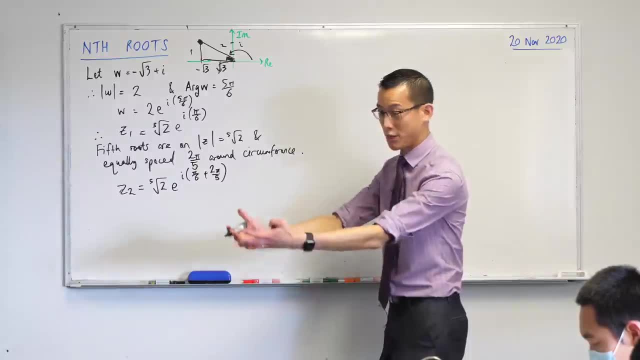 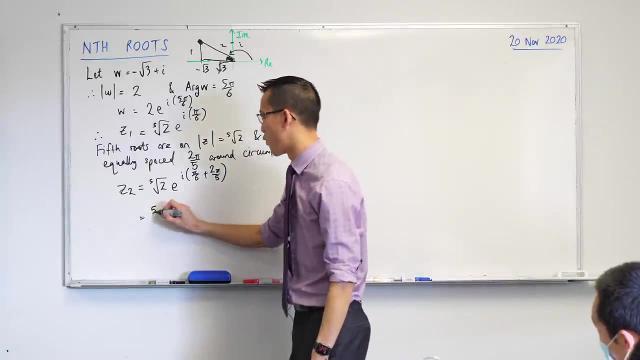 Okay now, at this point, I'm very happy for you to reach this point. reach for your calculator. Pi on 6 plus 2. pi on 5 is not the main thing we want you to focus on in this question. So if you want to reach for your calculator, don't worry about the pi's obviously put in a sixth plus two fifths. 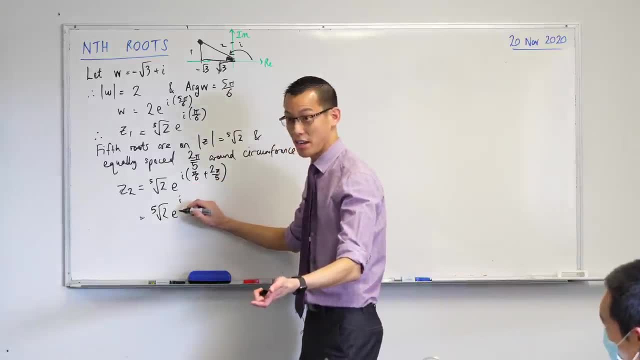 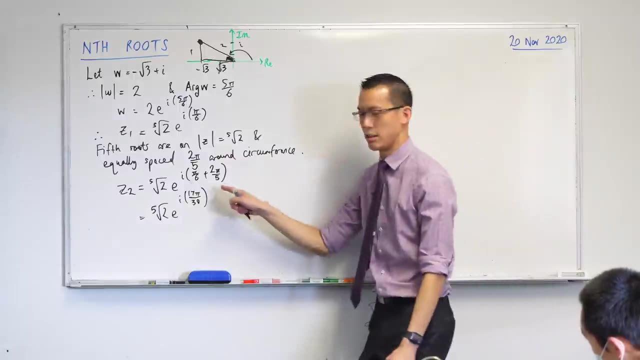 What do you get? 17 pi on 30 is what I remember getting when I was working this out earlier. 17 pi on 30, you should verify that. and you're like: oh yeah, denominator looks good, that's fine. 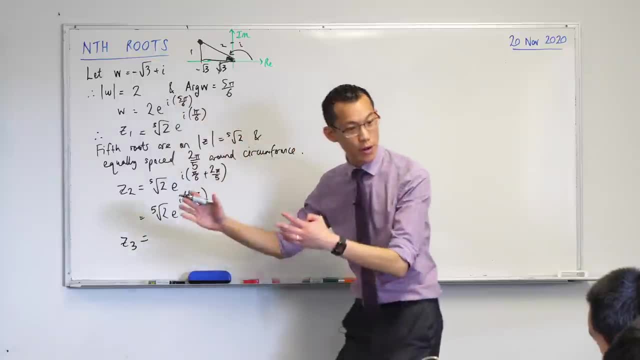 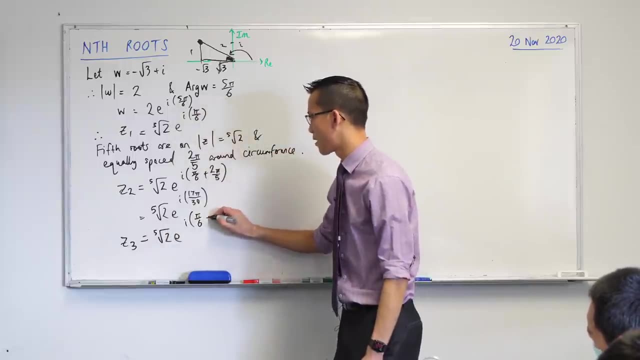 I've got my next one, z3,. I'm just going to go another 2 pi on 5, right? So it'll be fifth root of 2 out the front, e to the i same starter, but I'm going to go further, right. 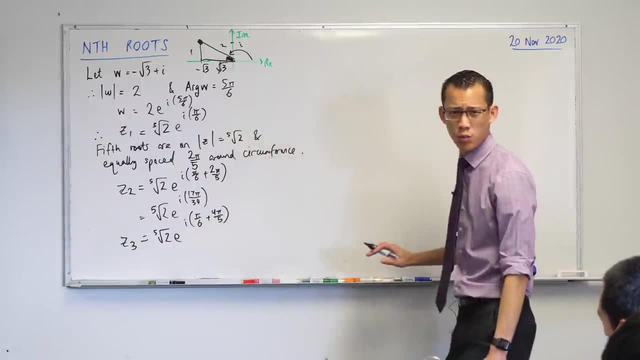 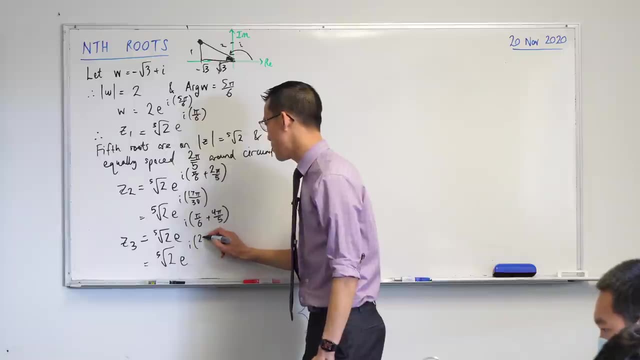 And calculator should hand you another answer From memory, it's 29 pi. Okay, now, at this point I just want us to pause. You're maybe settling in what did I say, 29? Maybe settling into autopi like this is great, like it's so. 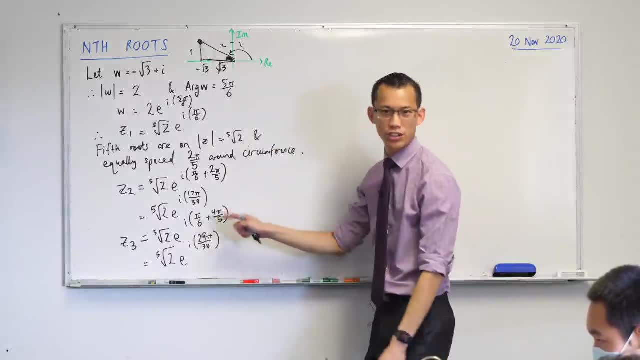 it's so well set up for us, the theory of it, that you can just keep going. You can go 6 pi on 5, and then 8 pi on 5, and then you'd be done. But just briefly, what I'd like us to do, even though it's not required. 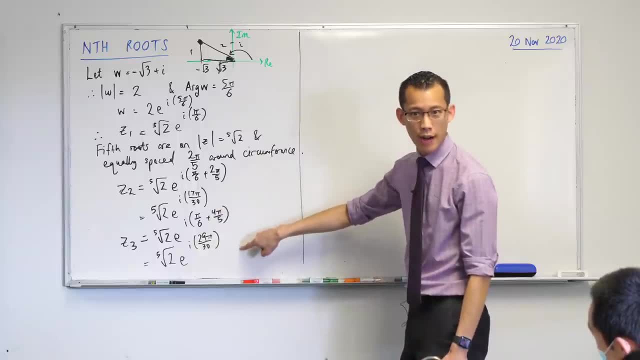 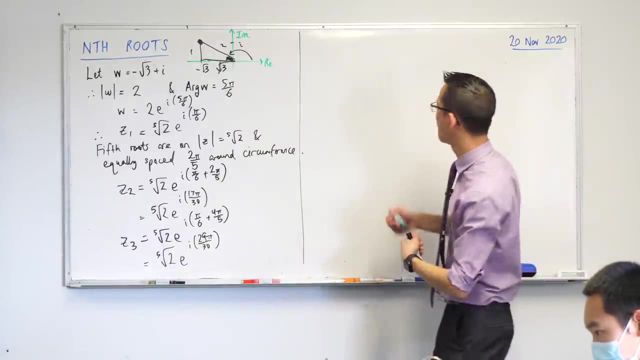 is. can we just quickly draw where these are on an argon-diagon, because this will be helpful for us in a second. If we draw, we're eventually going to get all five of the fifth roots. If we draw this on, you'll notice. 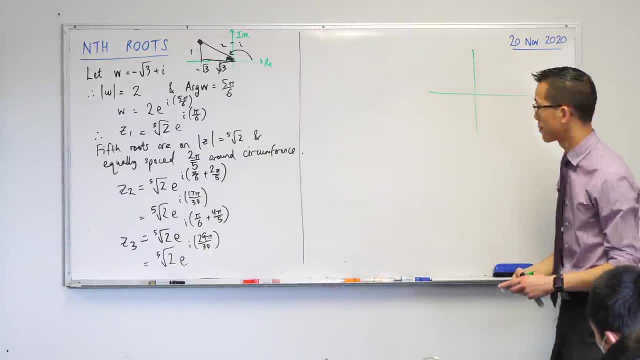 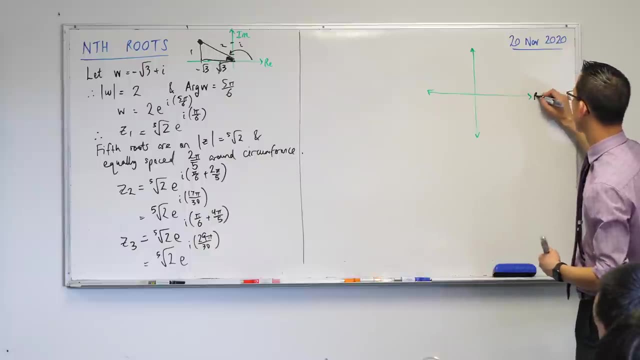 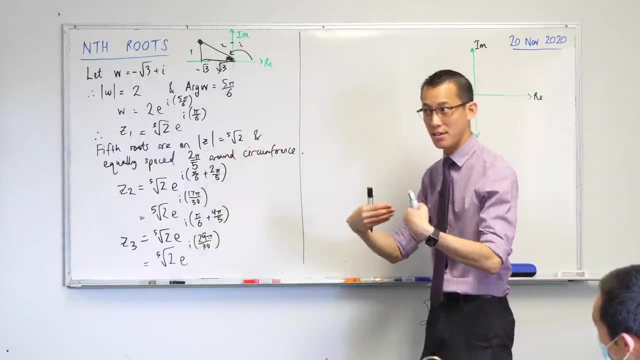 there's some geometry you can take advantage of here. Okay, so I'm going to draw my imaginary and real axis. Hold on to this one. Now my first solution, or sorry, rather, all my solutions, I know, are gonna lie on the circumference of this particular circle here. So just to make things easier for myself, 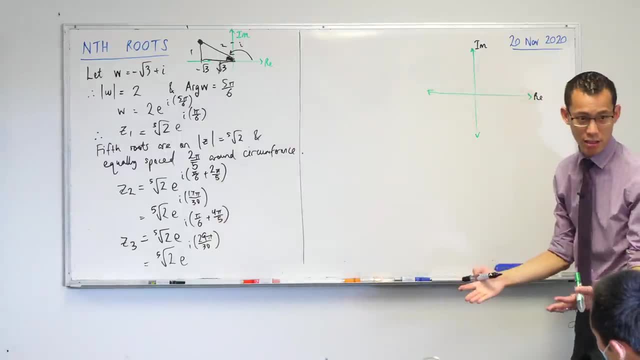 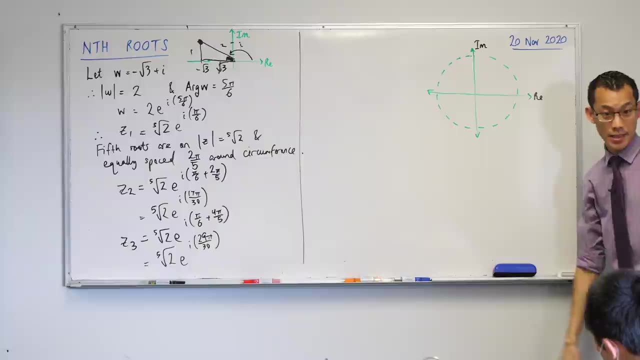 I'm going to put that circle onto here so all my solutions can live there, Okay? So I'm going to go ahead and, in fact, I'm gonna use this color. I'm going to go around. here's my, here's my circle. Okay, and it's. 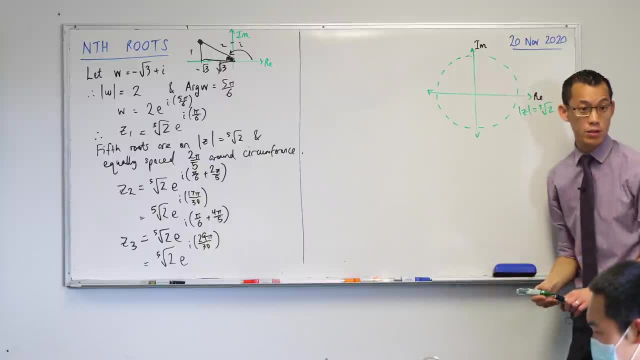 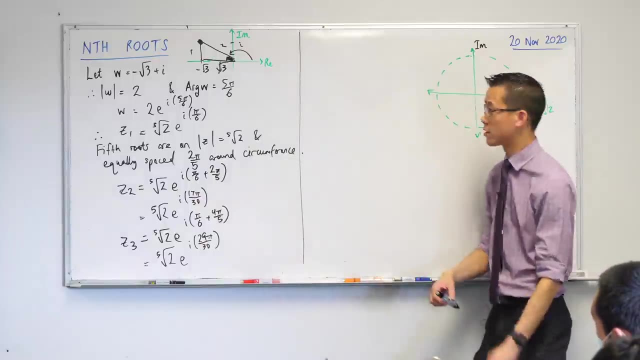 circumference, or its radius, rather, will be the fifth root of 2, so all my solutions will sit somewhere along that this circle. okay, and then from here i just need to know the appropriate angles. i've already got three of my solutions, so they shouldn't be too hard to plot. i'm going to place pi on six about. 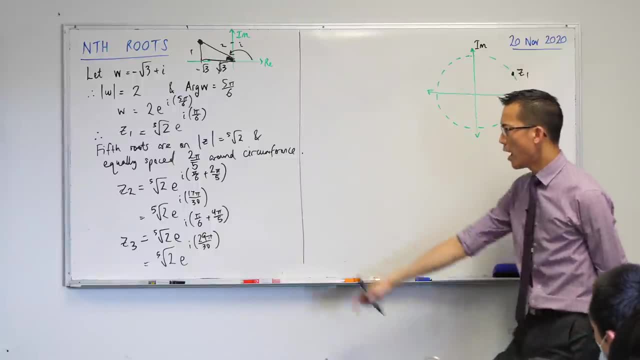 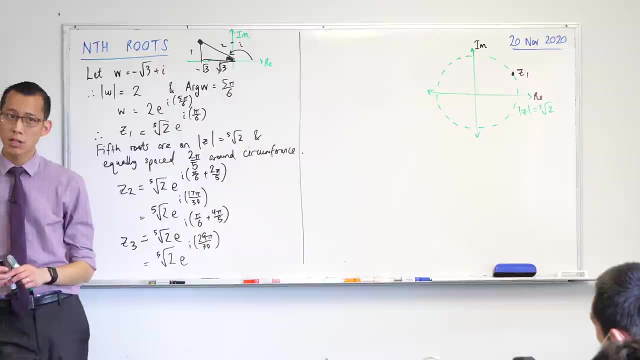 there. so this is z1. uh, this one here is z2: 17 pi on 30. now i just want to roughly get a sense of where that is. um, it's a little bit close to 15 pi on 30, right, just a bit further than 15 pi on 30. 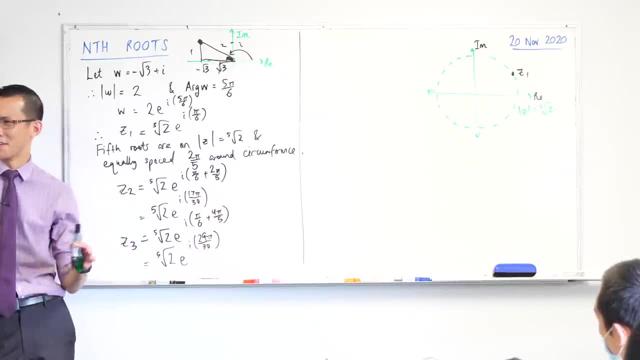 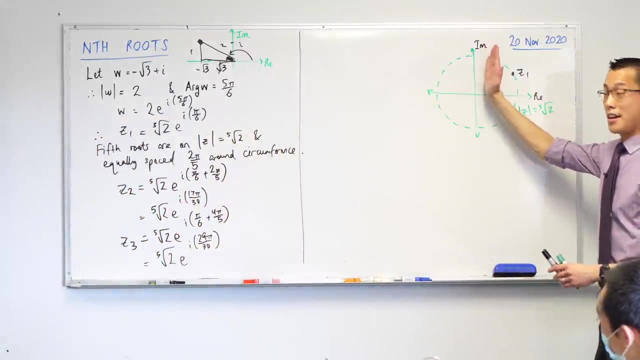 now, the reason why i think 15 pi on 30- like where that number come from- is what is 15 pi on 30 simplified to pi on 2, and i know exactly where that is. here's pi on 2. so if this is 15, pi on 30. 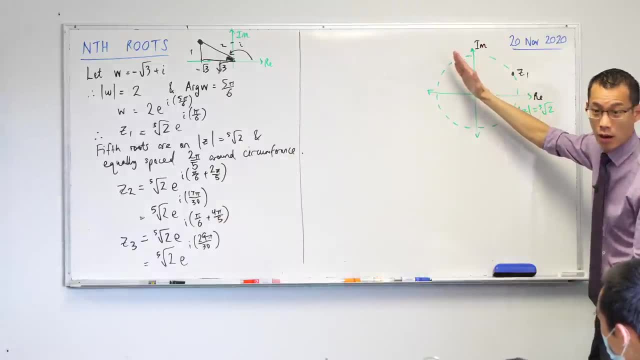 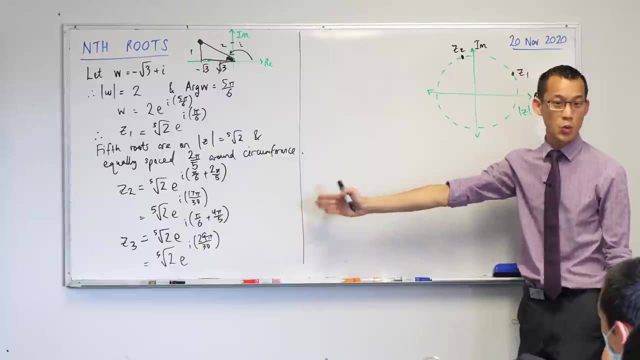 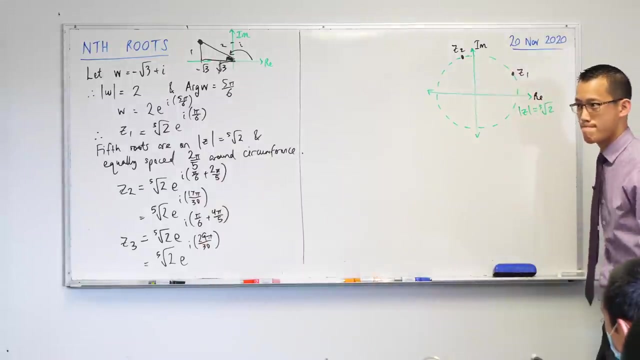 17 pi on 30 is just a little bit further anti-clockwise, do you agree with that? so i'm going to place that roughly here. there's my z2 and then my um. my third solution: 29 pi on 30. this is very close to 30 pi on 30. where is 30 pi on 30? on my ion diagram it's at pi, isn't it right? 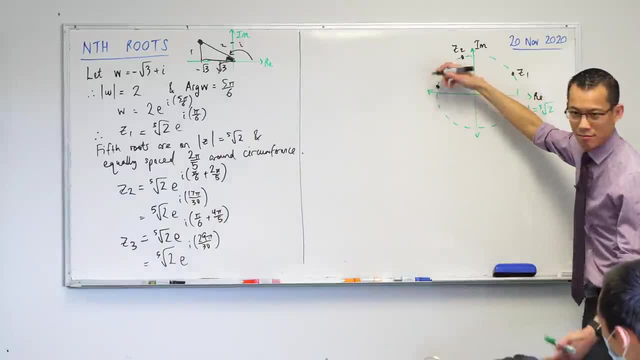 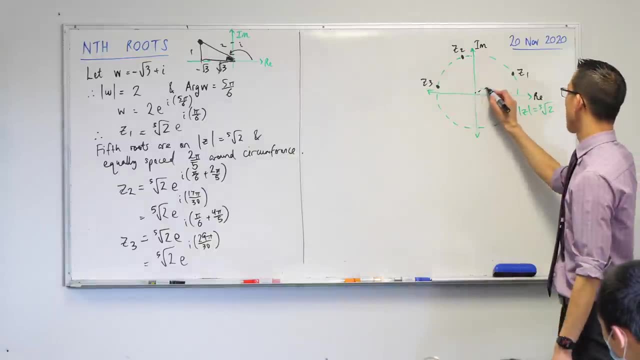 30 pi on 30 is pi, so i'm just short of that. there's ish 29 pi on 30, so there's my z3. so the way we've gotten our solutions so far is we've got our first one by using exponential form and then we got our others just by adding. 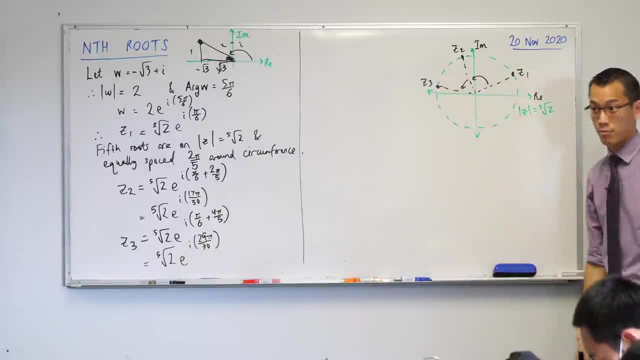 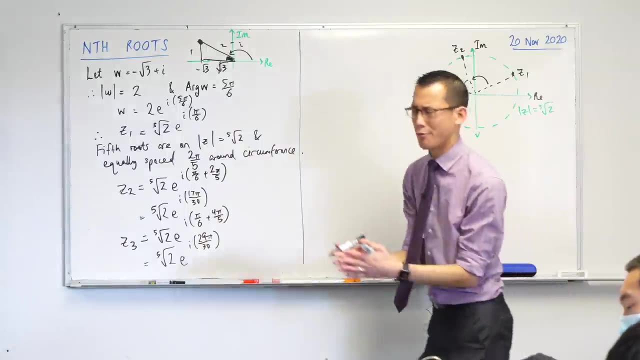 2 pi on 5 every time. does that make sense? and so we've arrived at our third solution so far. you can already see like we're going to get this um a regular pentagon, regular, yeah, regular pentagon. i was going to say regular polygon of five sides and realize i have a name for those. okay, i'm going. 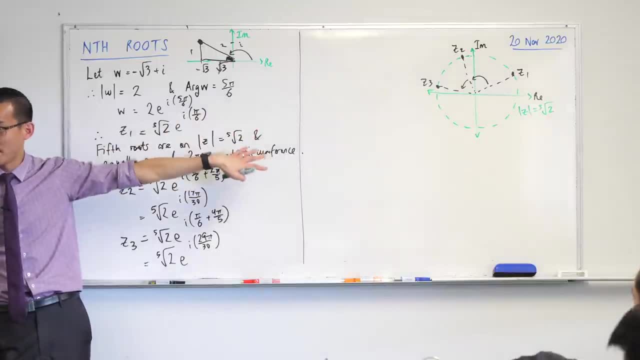 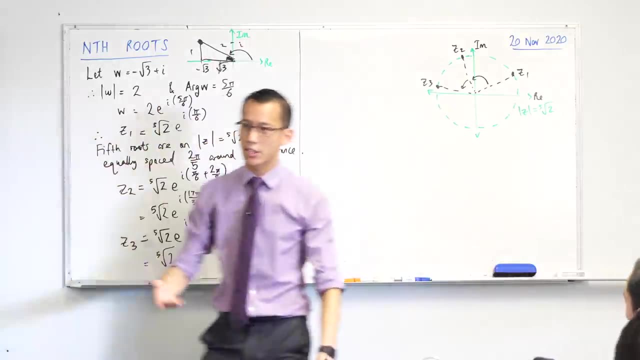 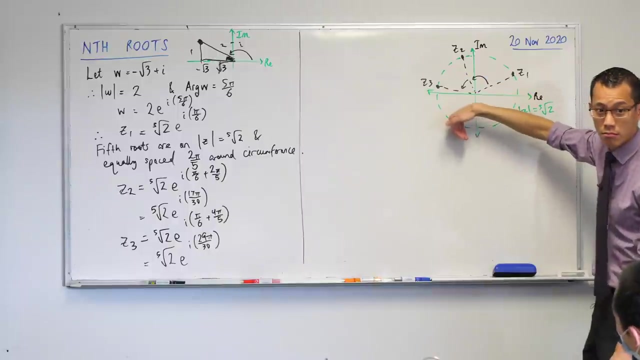 to get my regular pentagon. surely you can see i'm missing solutions down the bottom here. but at this point i recognize there's a better way to do this than to keep going anti-clockwise. if i kept going anti-clockwise i'd still get a z4 and a z5. it's fine. okay, but your angle is going to be past pi, right, so it's going. 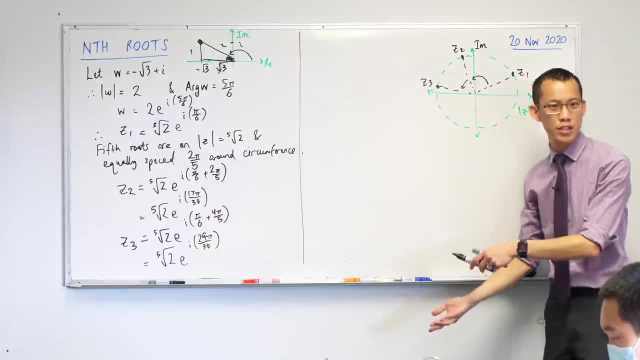 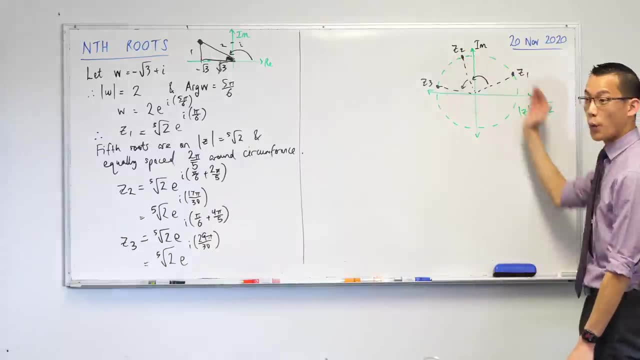 to be a non-principle argument, that's okay, you can change it into a principal argument, but why not just go for a? nor sorry. go for a principal argument in the first place, rather than continue going around. and you're going to get a z4 and a z5, and you're going to get a z5 and you're going to. 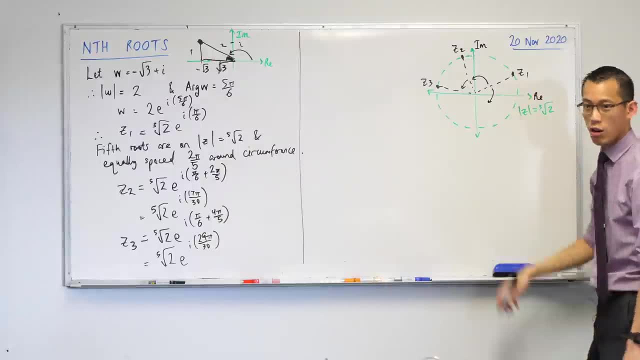 get an anti-clockwise. what if i were to go around clockwise? i'll still get these same solutions. it's just i can skip one step of converting to a principal argument. okay, so i'm anticipating- just looking at my diagram, right, i'm anticipating a solution around here and a solution around here. 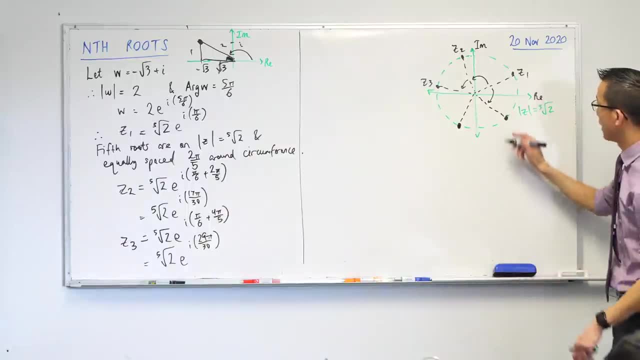 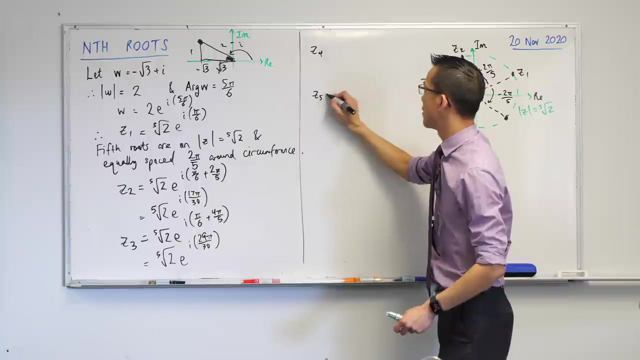 this will be my z4 and my z5. the difference will be: instead of adding two pi on five to go clockwise, i should subtract, so i'll. i'll give you a nudge right: my z4 and my z5. i'm still going to start from my first solution. 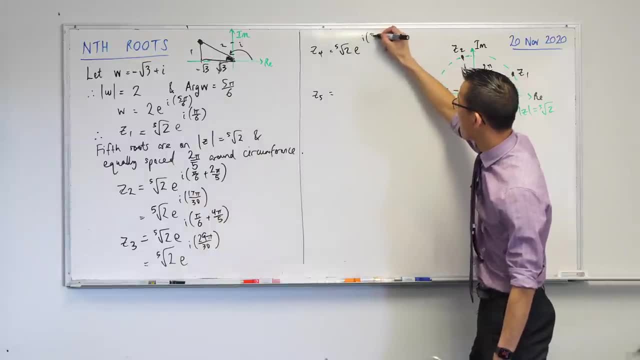 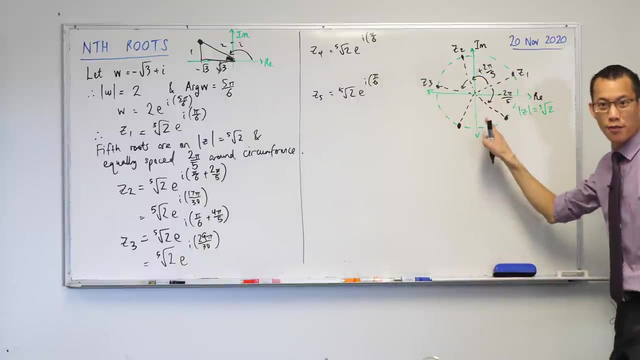 which in this case was fifth root of two e to the i pi on six, fifth root of two e to the i pi on six. but i'll subtract two pi on five to get this one, and then i'll subtract four pi on five to get the very last one. so that gives me this. 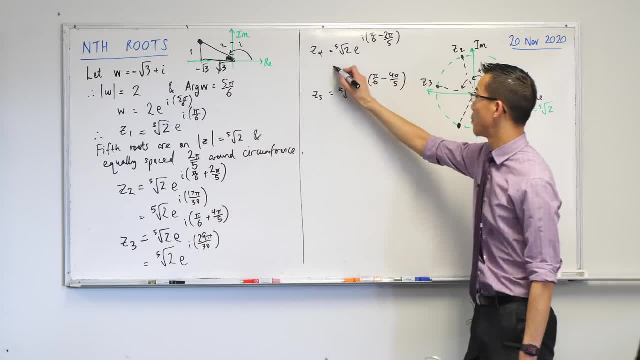 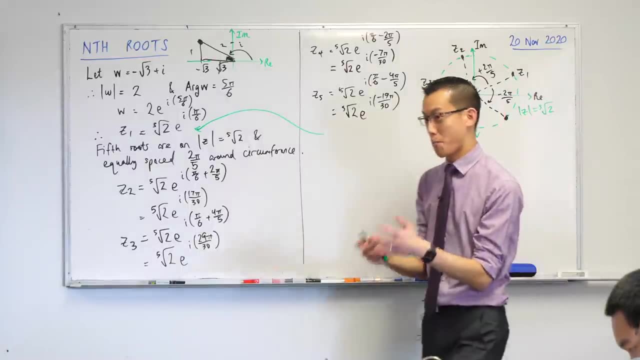 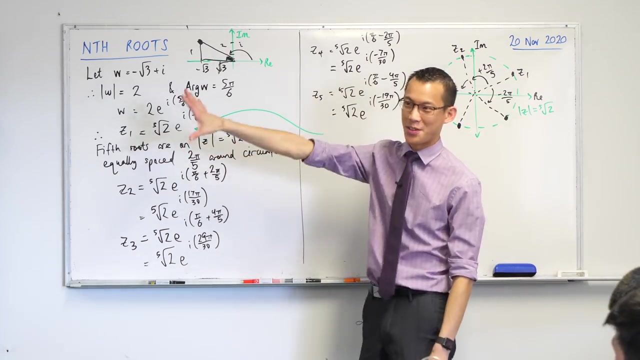 can you go ahead and uh work out what those are and then we'll um put them on the board together. all right, so we're, uh, we're, pretty much there, right? let me, uh let me, tie this up in a neat bow in two ways. for starters, here's one i prepared earlier, so this is obviously a lot neater than. 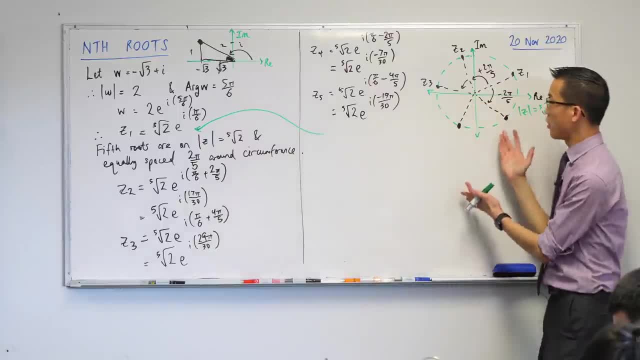 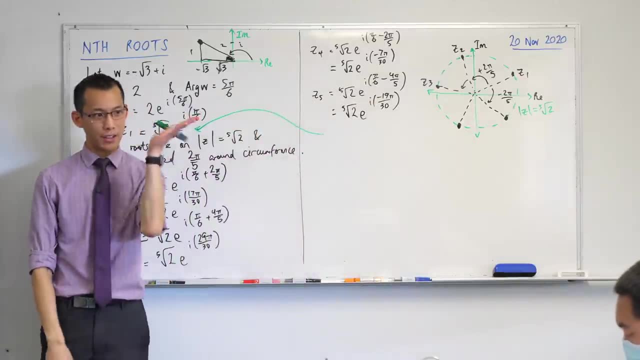 the one i did kind of in a hurry here. but you could already know you were going to get roughly the right thing, because you can see my regular pentagon forming there and you can also see how i got the first solution. went to two more and then went to the last two. 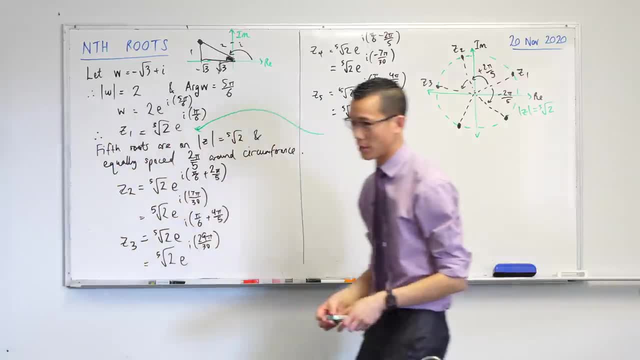 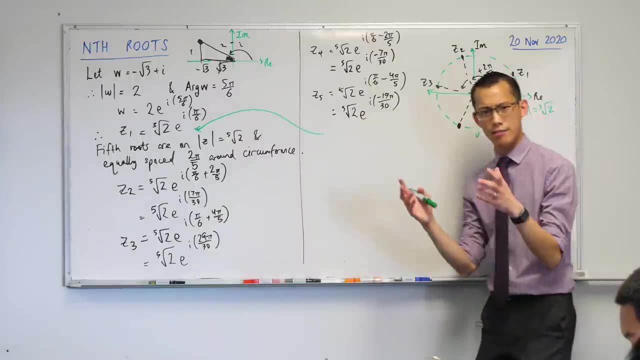 and so what it looks like in the first row. um, instead of two line structure, the first row has got a number function and all the lines are going in different directions. okay, now i should point out i sort of glossed over something real quick here and um lessons for. 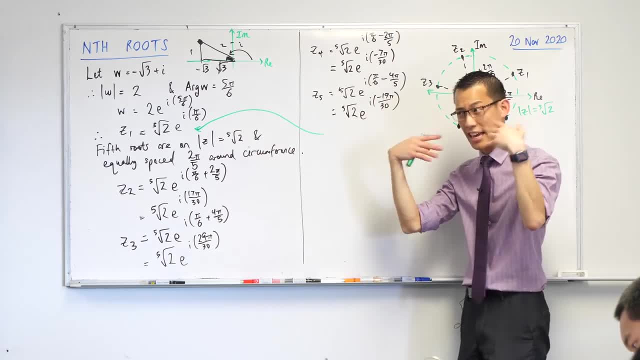 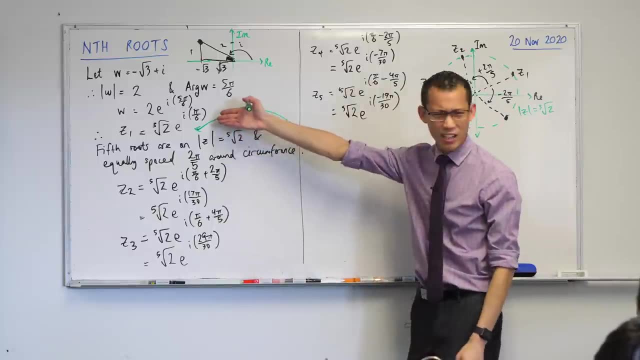 why you should not skip lines of working. uh, this is. you can see, like we've got you know. in our first question the focus was on complex numbers, but we had to use our trig identities and here we're still focusing on complex numbers, the complex plane, but i sort of snuck in index laws into here. 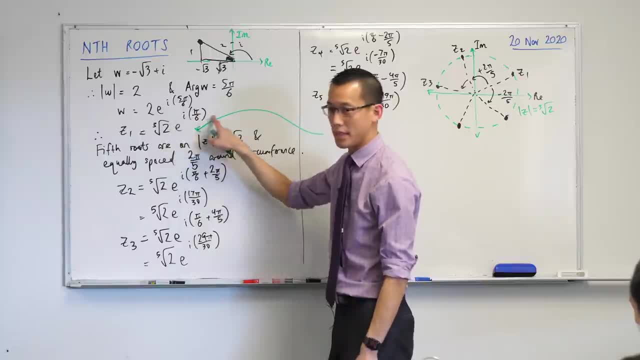 without really going into detail of why. so let me just put in one intervening line to hopefully make clear, even though it doesn't look obvious. right, we're doing the same thing over and over, but what's doing one thing to everything here, right? so let me write from w right if i write w, to the power of. 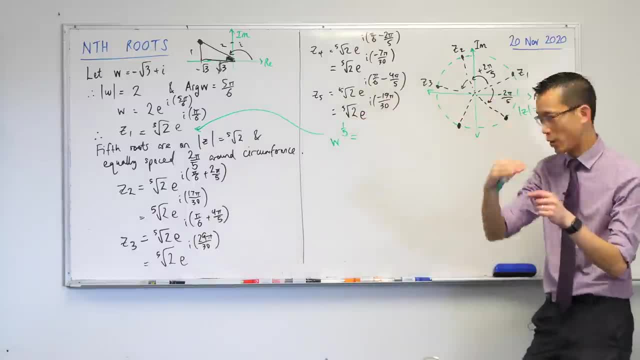 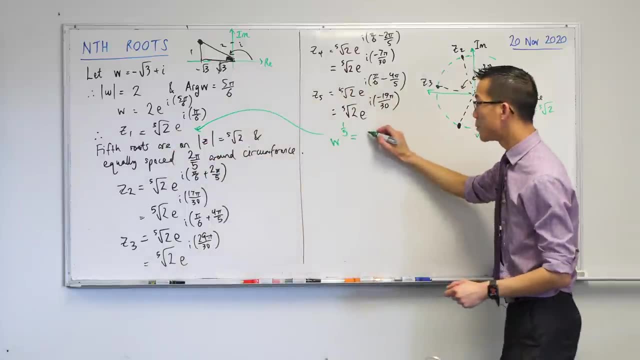 a fifth and maybe. um, for those of you who've already popped this working down just like, sneak it in on the side, just like i am, so you can really clearly get where this first solution is coming from. i'm just going to write everything in here and i'm going to raise that to the power of. 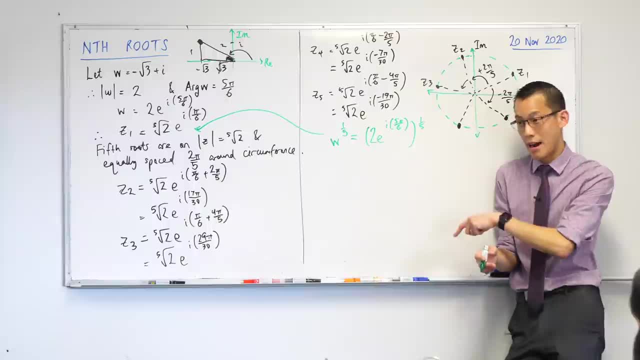 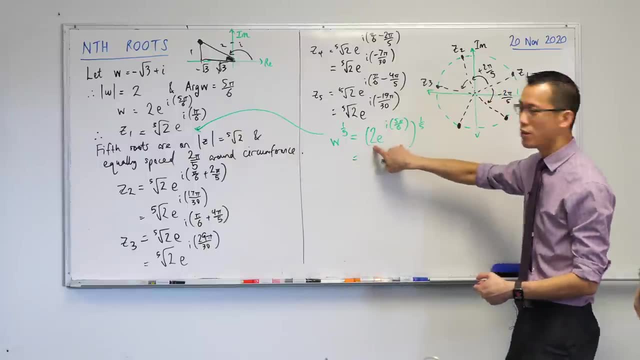 fifth: okay, so i did a lot of this index law stuff that we're about to write here kind of in the background because we get familiar with them, right. but for those of you who are like kind of i'm not quite there, you've got two numbers here: a product being raised to a power, which is the same.